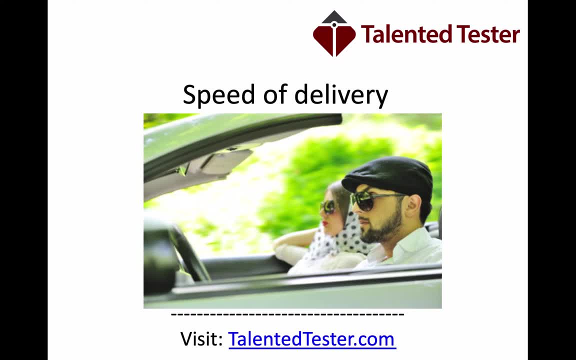 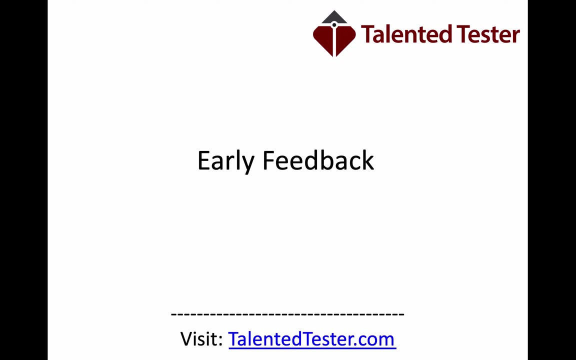 and getting early feedback, before you spend months of planning and designing only to find out that data It is no longer needed by your stakeholder or they just generally do not like what you've delivered. And, believe me, I've been testing for a long time now and I've seen this happen before. 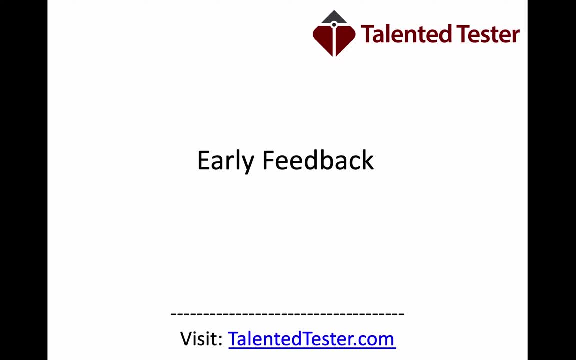 Early feedback falls in line with speed of delivery. You can roll out a few iterations. Let's give you an example. You could be building a graphical user interface for a web application rather than spending months on design and documentation and then maybe a month three. 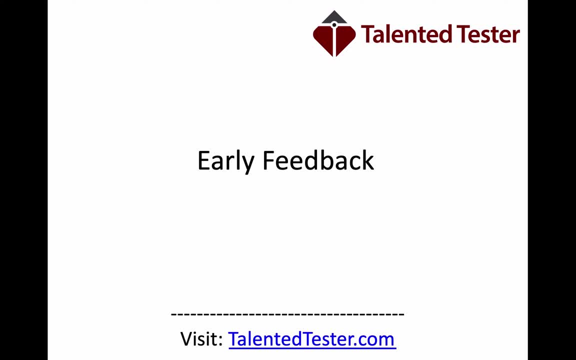 having a UAT testing phase, You could roll out the basic wireframe of the graphical user interface within one to two weeks. You can update your designs or code up related Doubles andTomatoes to be in line with your expectations and open problems. 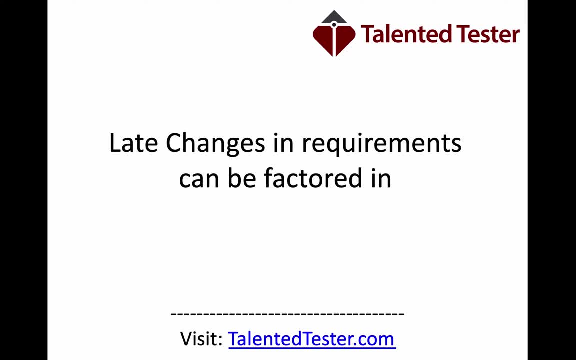 And you can reiterate this back in the next sprint. Last but not least, you can do some מה zach. Late Change, Later Change, Later Change, Late Change, Later Change, Later Change in requirements can be factored in. this is another great thing. agile is not as 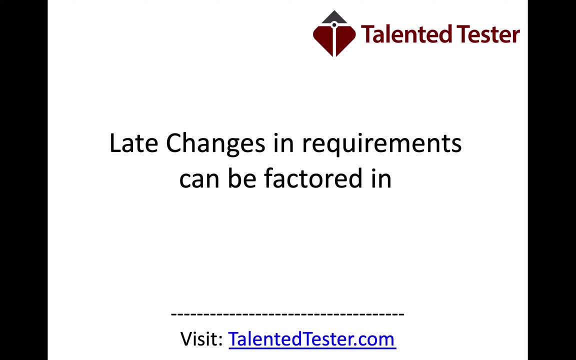 rigid as the V model or the waterfall model, so you do not have to go back to design and documentation. if there is a change in requirements and have loads of meetings to agree the changes, you can simply tweak the changes, add it to the next sprint, redevelop the code, update the code? what or have you? whatever it? 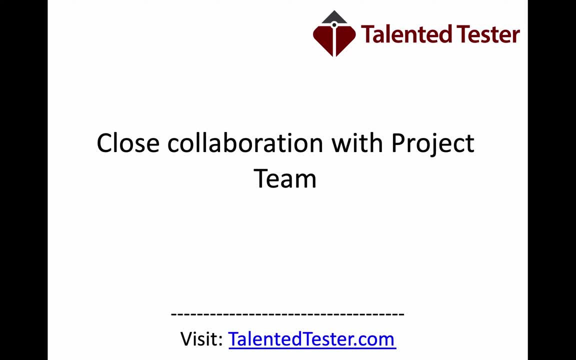 may be retest and then roll it out. close collaboration with project team. one of the benefits of this is you can collaborate closely with the project team and it allows the buy-in from all people. in a project team, for example, you'll have the project manager can have a good view of the next sprint. the 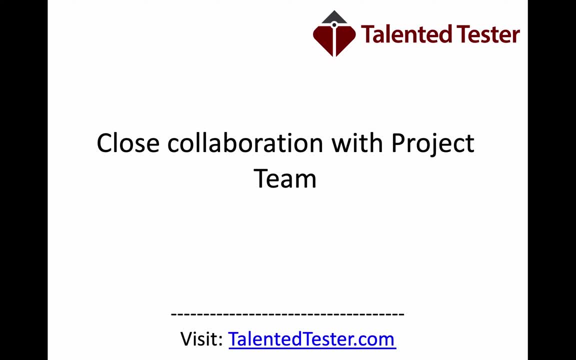 stakeholder can get some feedback on the sprint and at the end, before it's actually, you know, too late to make changes, and it's a good opportunity for test the development developers and all stakeholders and project members to collaborate tightly together. one of the great things in agile, which is known, is a scrum and this: 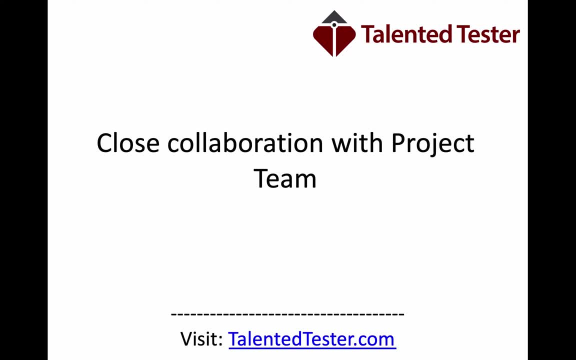 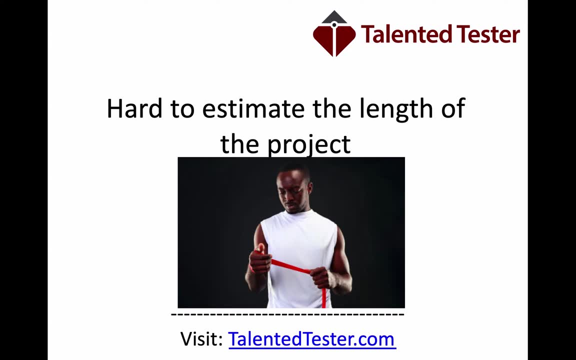 is an opportunity for all stakeholders to get together on a daily basis to see how the project is unfolding. now, one of the disadvantages is it's hard to estimate the length of the project now, depending on how you implement agile, because every company has their own flavor of how they actually implement. 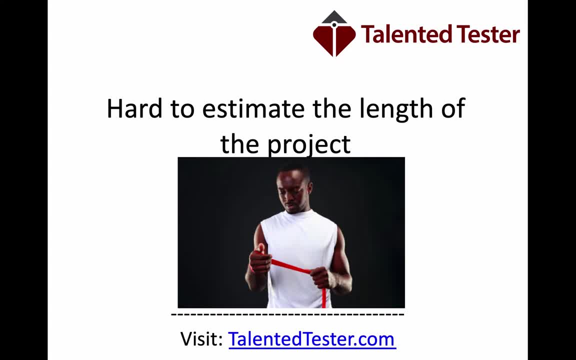 this regardless of what you may have read in a book. every company does it slightly different and, being in the game for just over 18 years at the time of recording, I've seen it. I've seen many different flavors of of implementations of agile. sometimes it's very hard to. 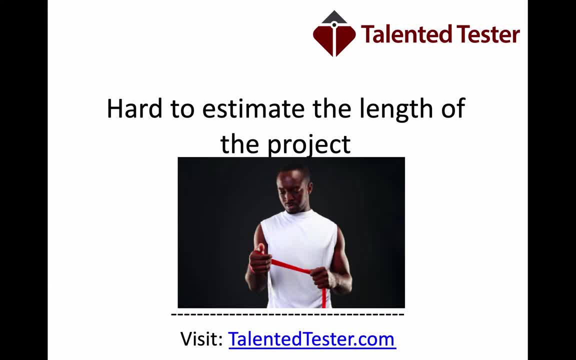 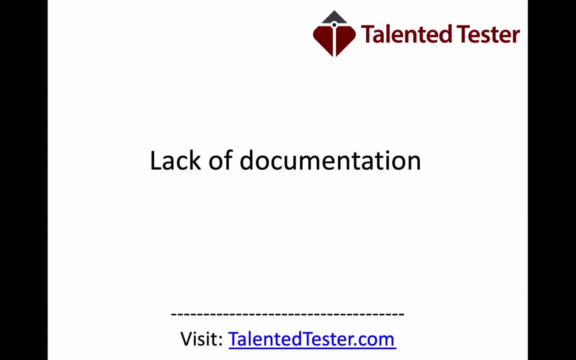 estimate the length of the project, because there is a tendency to continually add new sprints and modules and never really have a known end date- lack of documentation. now, if you're traditionalist or someone that's worked in the game for quite a long time and you've used models such as the V model, 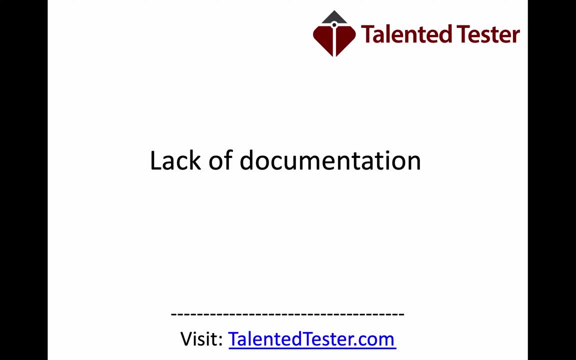 and anger, you can find a lack of documentation and that are quite hard to actually deal with, and it's something that is seen as a negative, but it's a matter of opinion, actually, because some people believe this is a bonus, because they don't have to get bogged down with months of planning and then filling out. 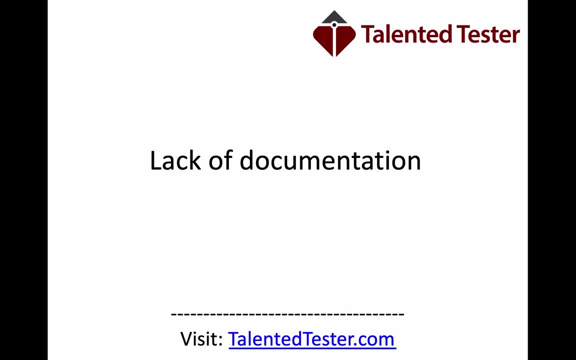 documents rather than using that time on getting feedback from their clients. so an advantage for some, but in my opinion, a disadvantage is the lack of documentation. scope creep: if you you've been testing for a little while, you've probably heard of scope creep before. scope creep in general is when you have some agreed requirements. but 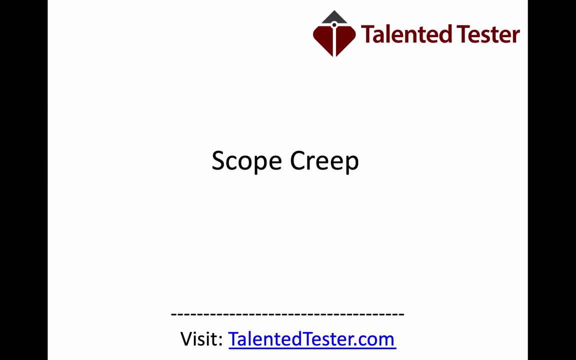 then you find, over time you start to go outside those requirements and you start to deliver something slightly different. sometimes this can actually be a gift, but it can also be a curse, because you can end up spending more money on the project than it was expected and delivering something which is slightly 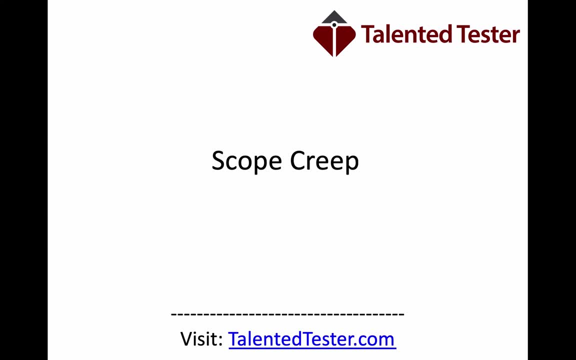 different to what you've agreed for, and this can be quite a costly mistake. in agile, it's very easy to do this because it's so flexible. you don't have the entire scope nailed down from the beginning, so it's very easy to go off on a massive tangent. when should you use? 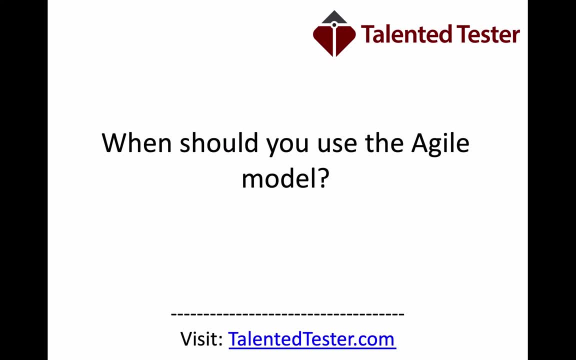 the agile model, and that's a very good question. in my opinion, the agile model is really good for projects where you want fast delivery, something which needs feedback really quickly. it's ideal if you've got a web application that you can get feedback from your client, update and go forward if it's a more complex 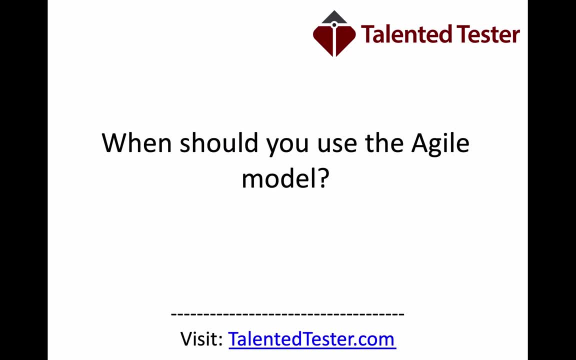 financial application. it may be debatable if this is the best model for you. I'm not saying it's not being used in applications like this before, because I'm sure it has. but the big thing is, if you're using agile and you've got a very large team, which